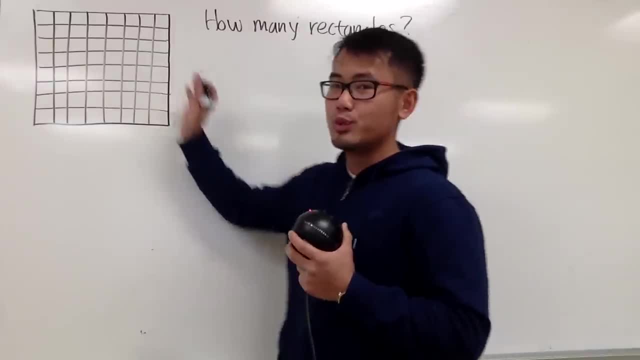 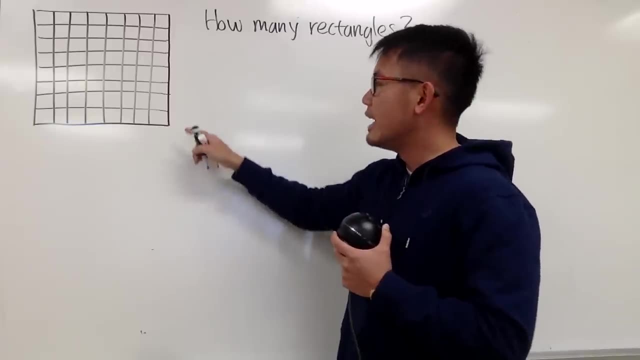 Okay, let's do some math for fun. Here we are going to count how many rectangles do we have right here? And this is meant to be an 8 by 8, like a chessboard or like a checkerboard. okay, And keep in mind, this is meant to be a square and each square is a rectangle. 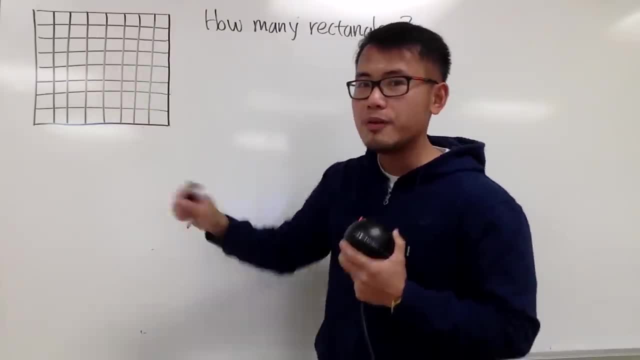 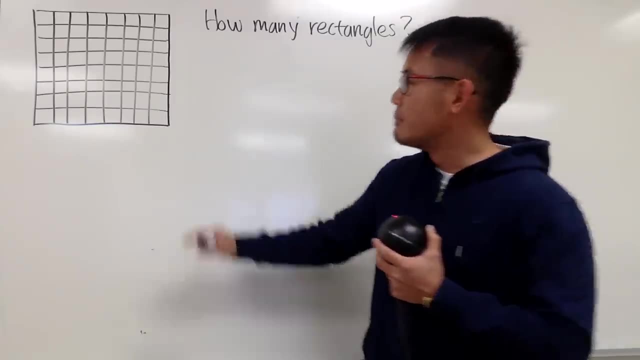 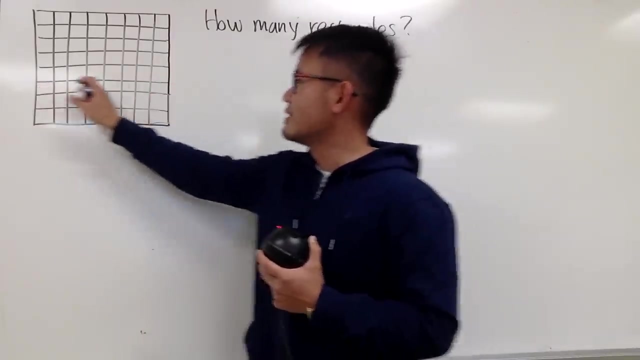 So by just looking at this picture here, we have a total of 8 times 8, namely 64 little squares. So that's 64 little rectangles. But remember this: right here it's also a rectangle, So it's one whole row like this. It's of course not a rectangle, right. 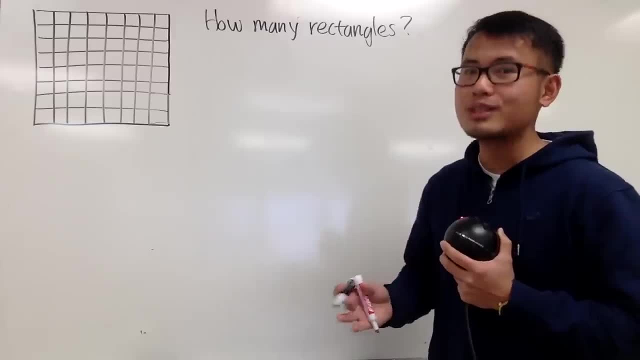 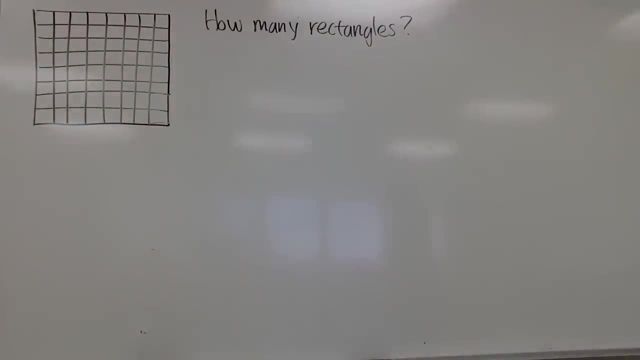 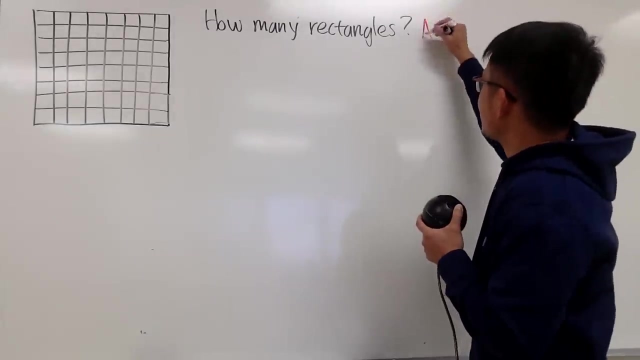 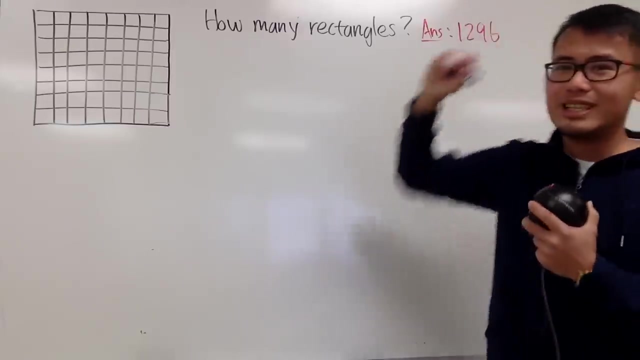 So the question is: how many rectangles do we have right here? As always, please pause the video and try this first. Okay, the answer to this- and let me just write it down right here- is: we have a total of 1,296 rectangles. 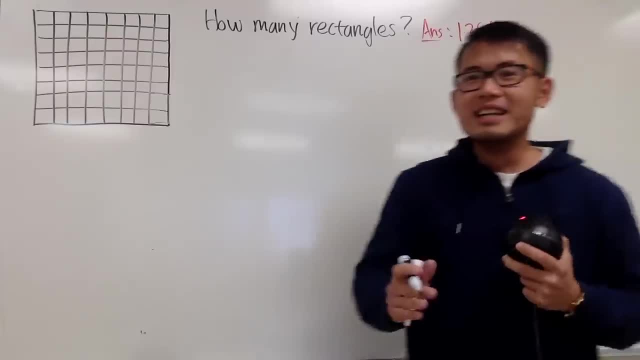 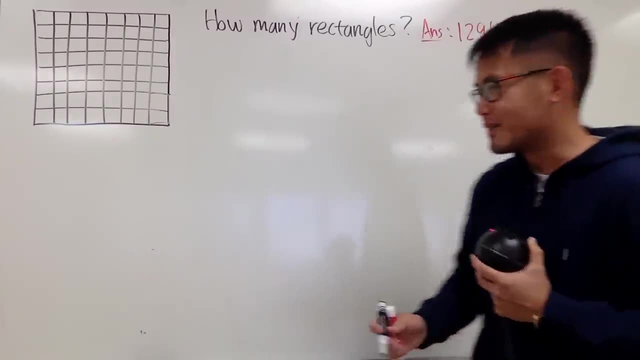 No more, no less. This is it. And if you just count, right, just seriously, just count how many rectangles there are, I think you might be still counting right now, right, Maybe after I finish the video in like 10 minutes or so, you're still counting. 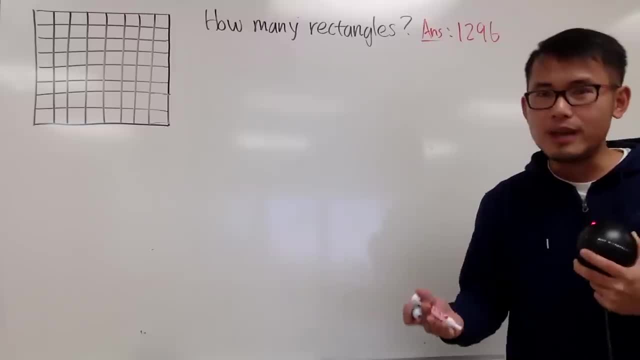 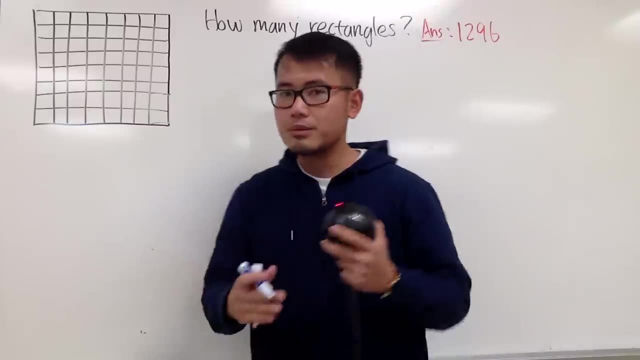 But you know, we are going to see if there's any efficient way to figure this out rather than just count. Here is the answer, Here is the first strategy. alright, The first strategy is that I think in the computer science they just call this divide and conquer. 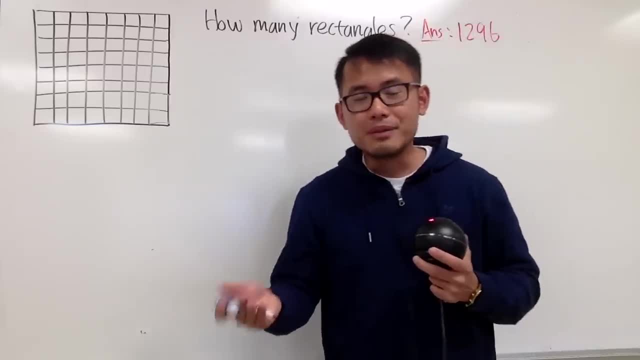 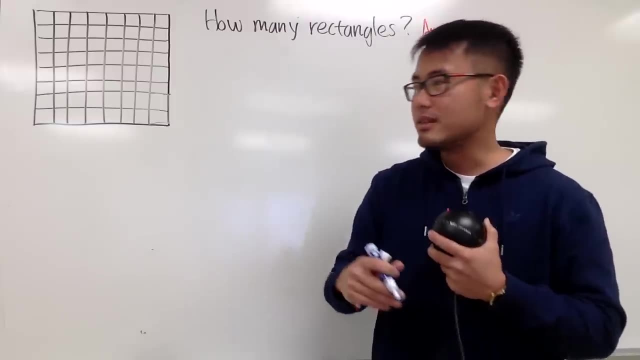 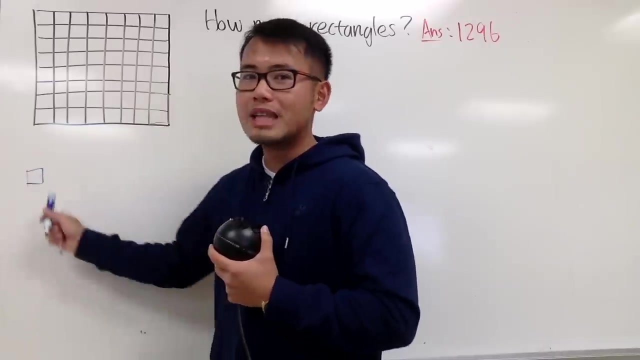 Maybe it's like this, But in math, one of the problem-solving strategies is that when you are dealing with something hard, let's consider something that's easier, something that's much more doable. Consider the smaller cases. So let's see what if we just have, one by one. 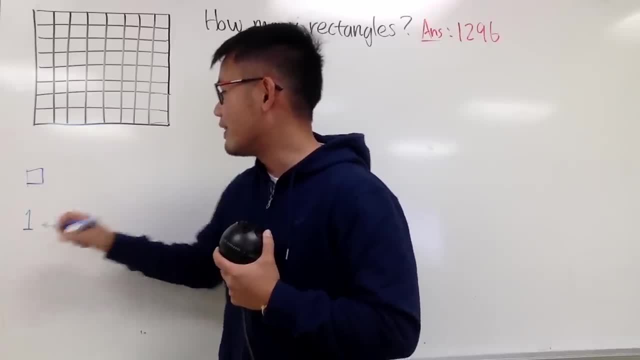 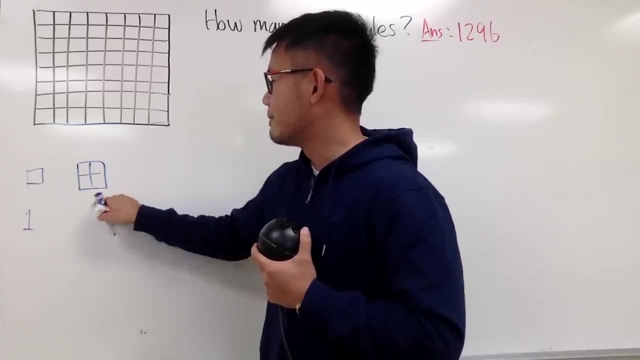 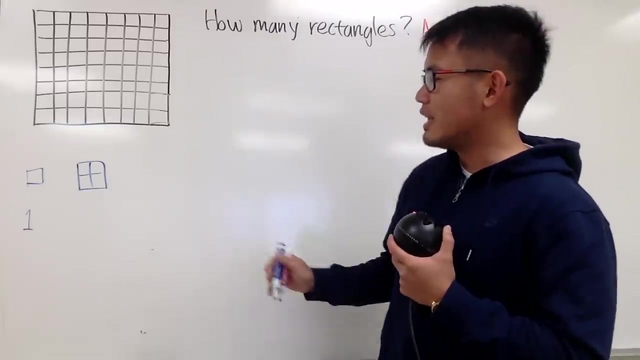 Of course you can just count this easily. We have one rectangle right here, right. And now what if we have a two by two situation? So you consider some smaller situations and hopefully maybe there's like an answer, like there's a pattern for the answer that you can figure out. 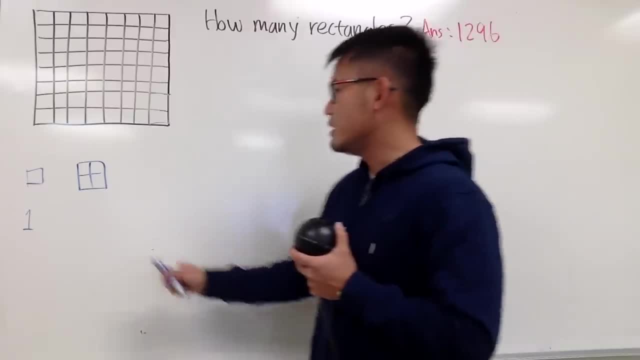 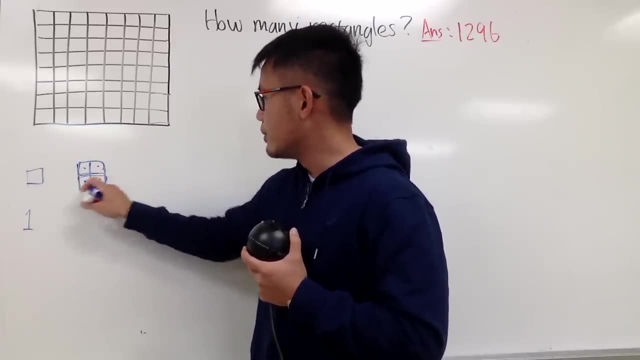 If that's the case, that would be so wonderful, isn't it? And let's see, let's just count. This is going to be one, two, three, four, And then one, two, three, four, So total of eight, right. 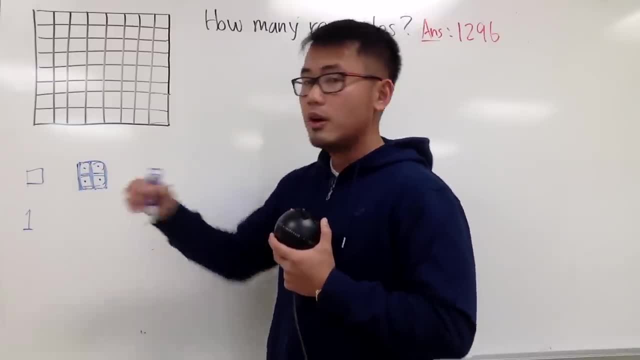 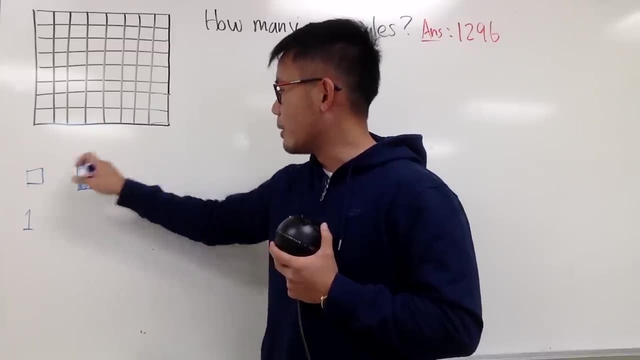 Four of the little ones and then four of the- you know, the longer ones like this. So now I have eight And keep in mind we also have the one big one, so we have a total of nine of them, right? 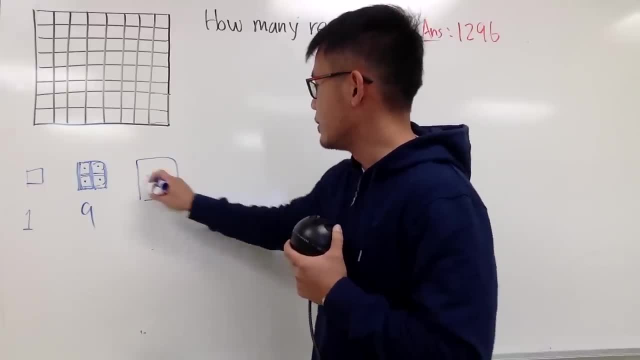 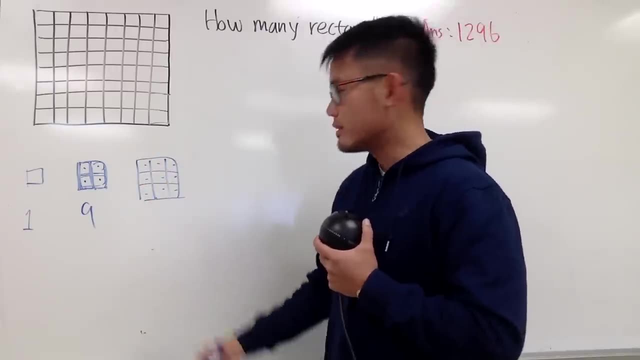 And now we'll just see. let's see if we can do the three by three situation. So one, two, three, four, five, six, seven, eight, nine, right? So we can just remember that this is seven by nine, for now. 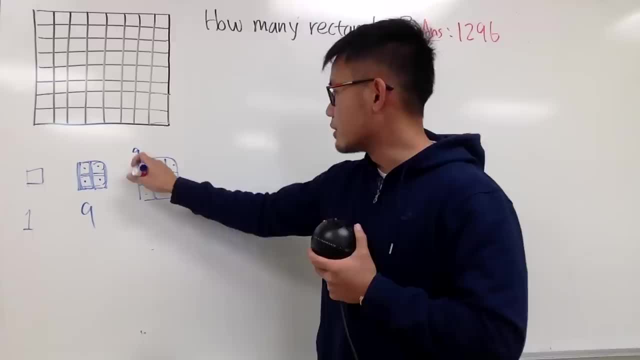 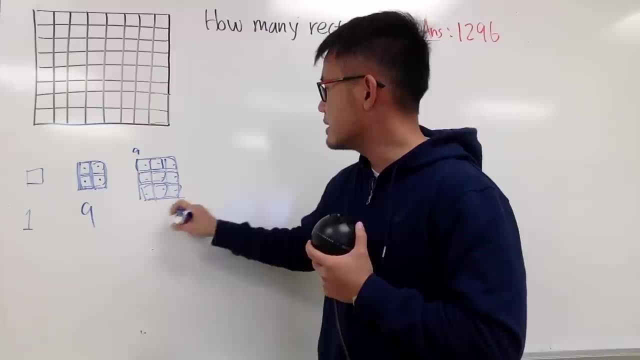 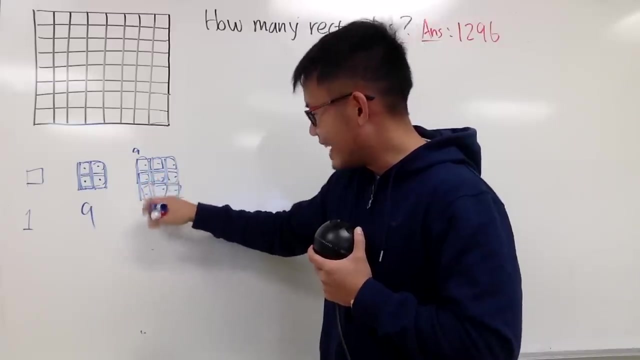 And then let's do the two by ones. So I'll just say this: One, two, three, four, five, six, and then let's do this way: Seven, eight, nine, eleven, I mean ten, eleven, twelve, right. 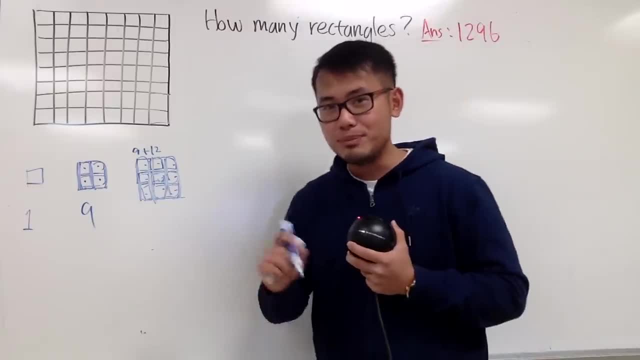 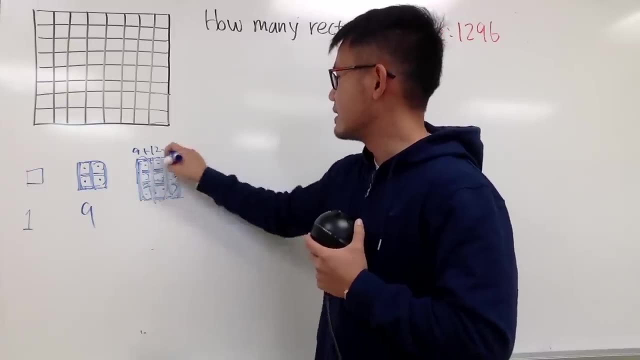 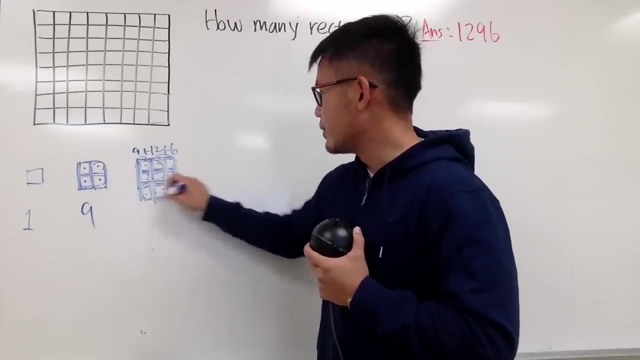 So we put down plus twelve, And now let's do the three by one: One, two, three, four, five, six, right? And now let's do the Two by two, right? So this is one, two, three, four. 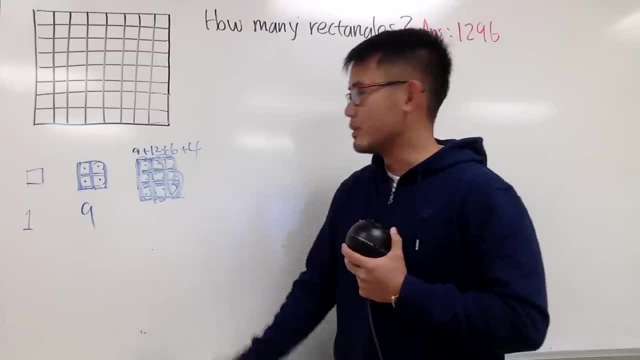 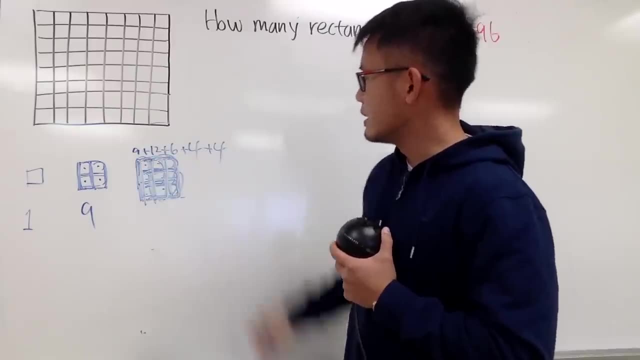 So that's the two by two, And now let's do the three by two. Three by two, we have one, two, three, four. So yeah, So we did the three by two, We did the three by one. 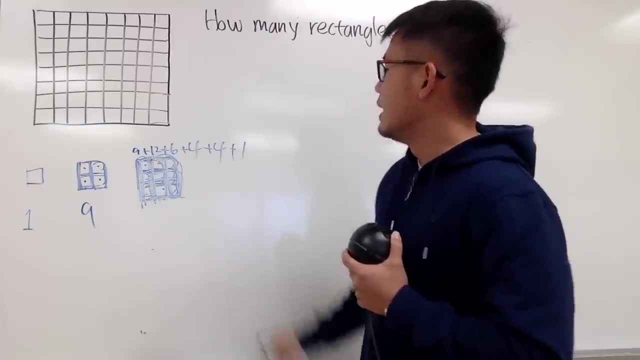 Now the last one is just three by three, So the last one is just this, So plus one, And of course we can just add this up real quick, And if you add them up, this is ten, This is another ten. 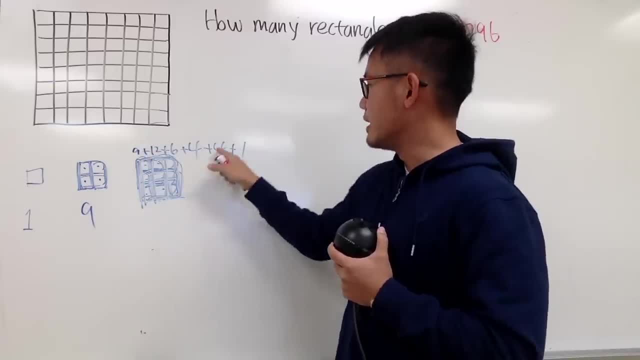 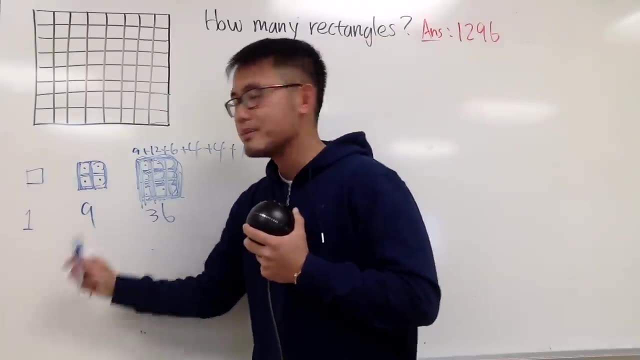 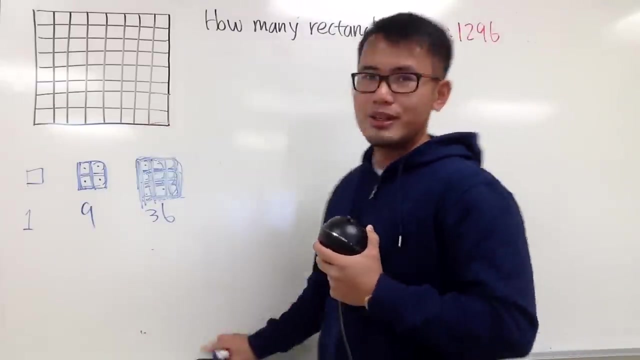 That's twenty, So we have thirty-two and then thirty-six. So, based on the first three cases, we have one rectangle, nine rectangles and then thirty-six rectangles. okay, All right, Let's see if there's any pattern for this. 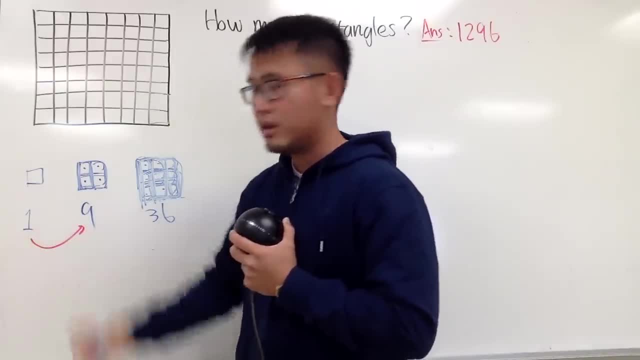 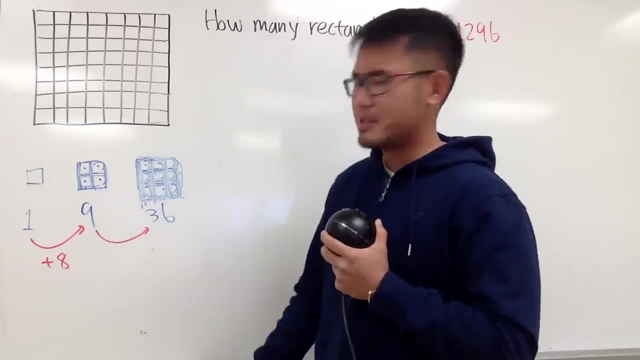 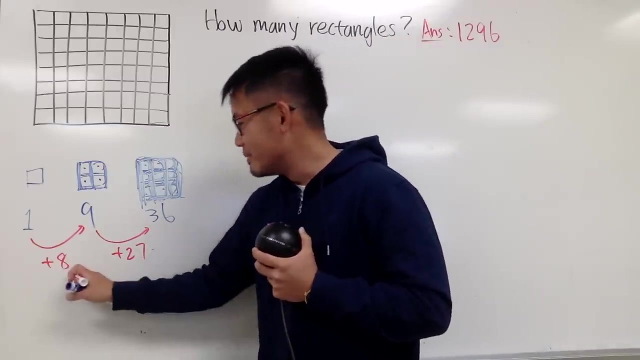 How can we go from one to nine? Well, that's plus eight, right? And how can we go from nine to thirty-six? That's plus twenty-seven. And do we recognize these numbers? We should, because this right here is precisely two to the third power. 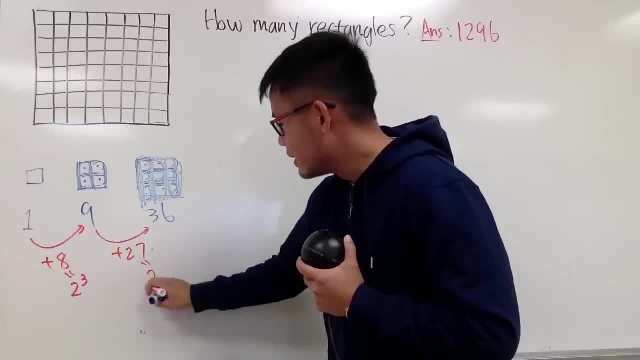 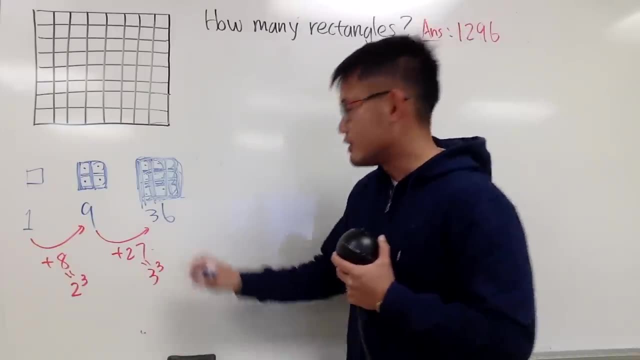 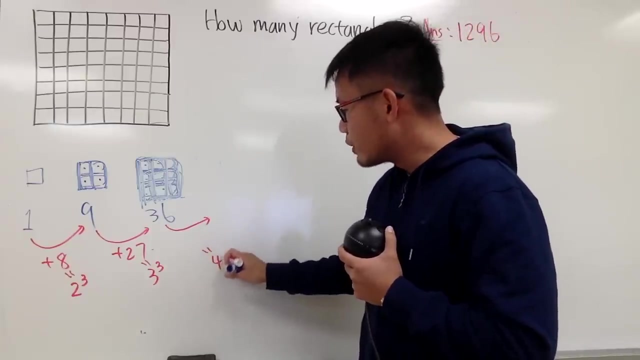 It's a perfect cube. This right here is precisely three to the third power. right, That's also a perfect cube. So you can imagine. what number do we need to add next? Well, we must add four to the third power. 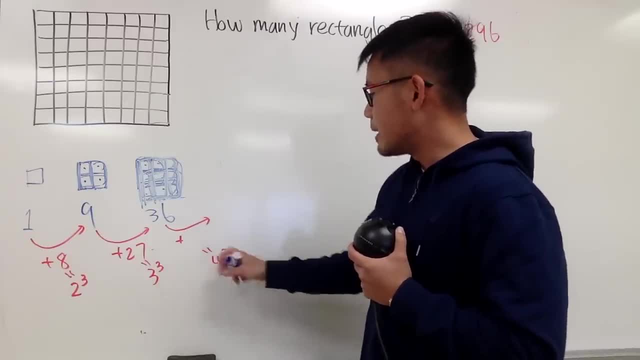 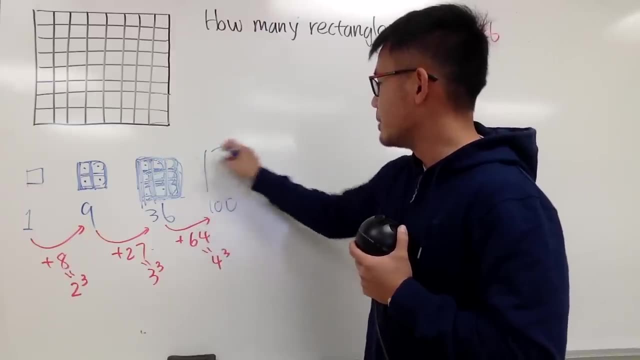 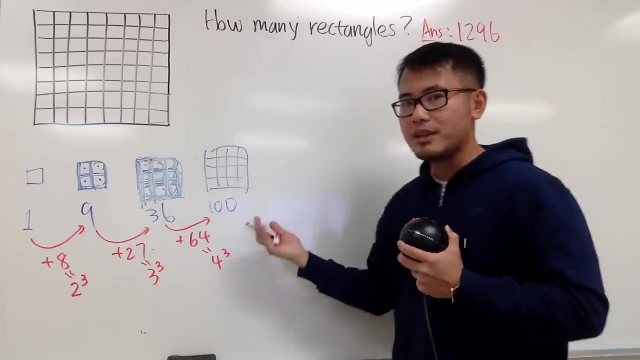 It seems like it. And four to the third power is going to be sixty-four. Thirty-six plus sixty-four, we get one hundred, And that's going to be the number of rectangles in a four by four situation, And I'm going to leave it to you guys to verify this on your own, all right. 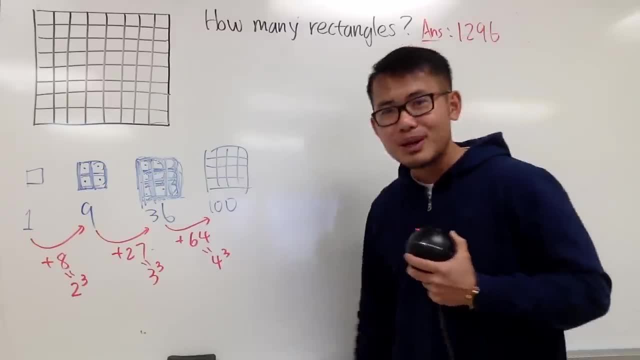 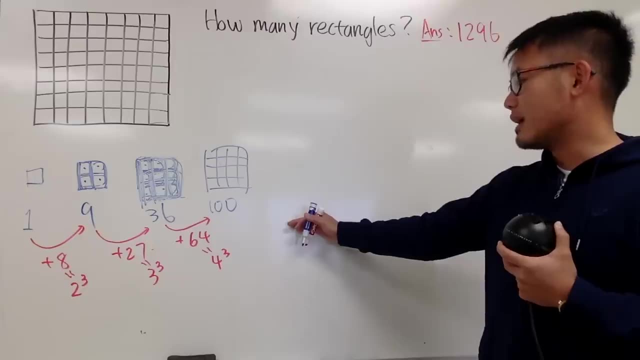 Because one hundred. I'm not going to show you guys how to count up to one hundred, All right. So this is kind of cool. And the next one, we can just go ahead and do plus five to the third power, and so on, so on, so on. 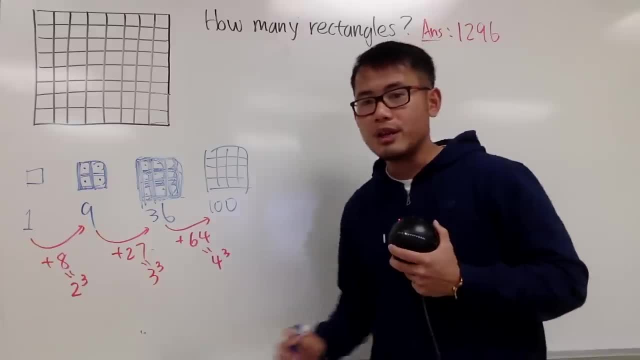 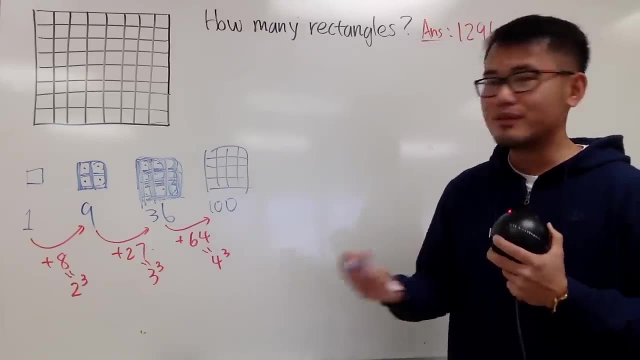 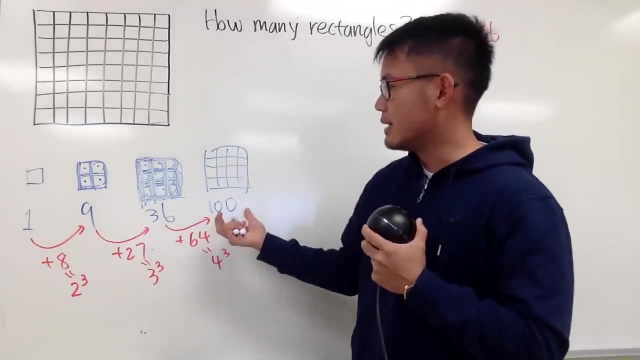 I do want to make a remark before we continue anything else. This right here it seems legitimate, but you know it's still not perfect in the sense that we don't have a proof for it. Sometimes you cannot really judge the numbers, the pattern, based on the first few cases. 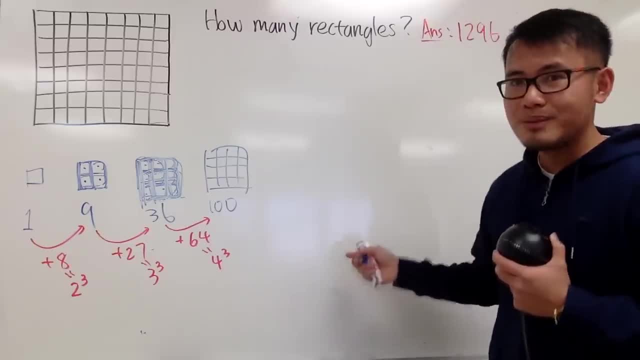 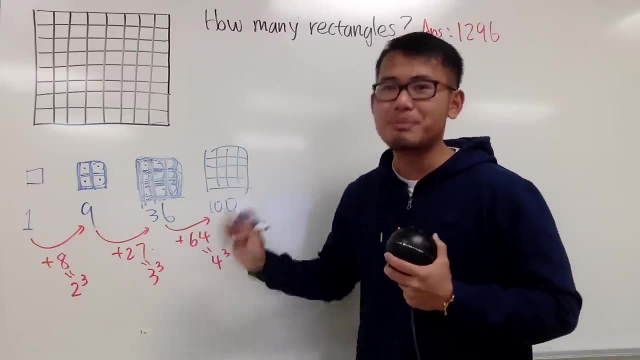 Sometimes the pattern may be broken later on. That's why we have the mathematical induction, all right, But at the moment, just trust me That this is actually the correct pattern, all right. So, anyway, this is the four by four situation. 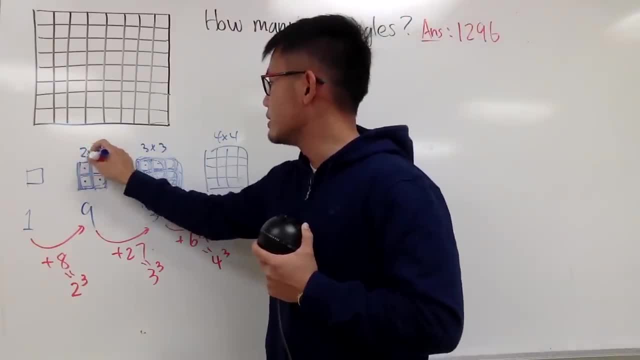 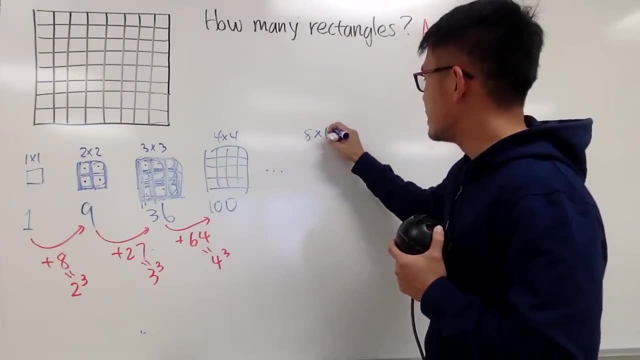 Let me just write this down for you guys real quick. all right, So this is the nine situation And of course, dot dot dot And we are going to get to the eight by eight situation, And of course you can just draw the rectangle. 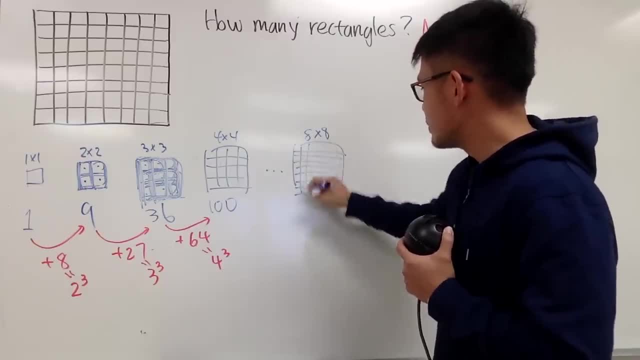 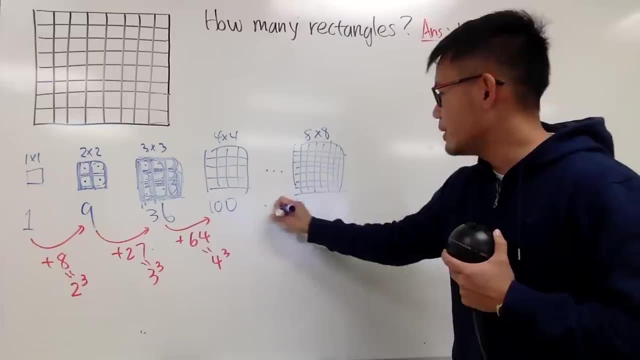 One, two, three, four, five, six, seven. One, two, three, four, five, six, seven. It's more than five. you know And just pretty much do the following, So I wanted to know what this is. 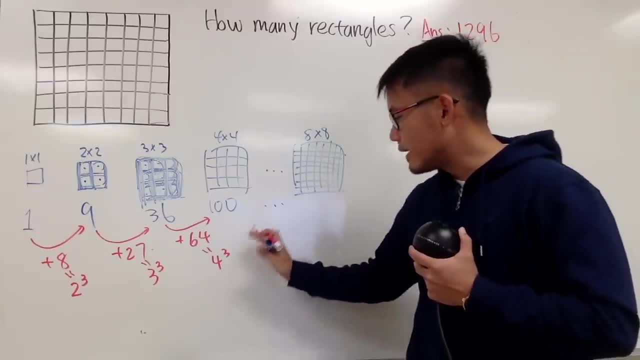 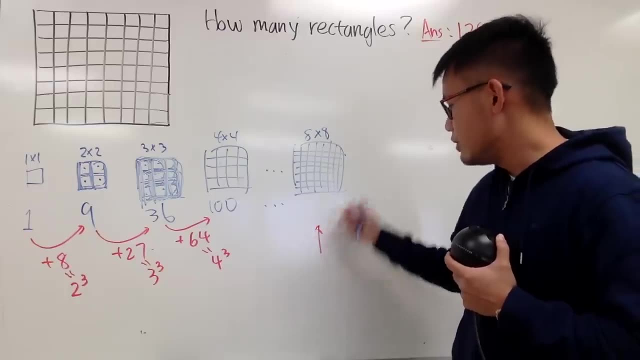 Well, the next one is going to be plus five to the third power, right? So once we get to the eight by eight situation, this right here it has, it should be one to the third power, because that's one right. 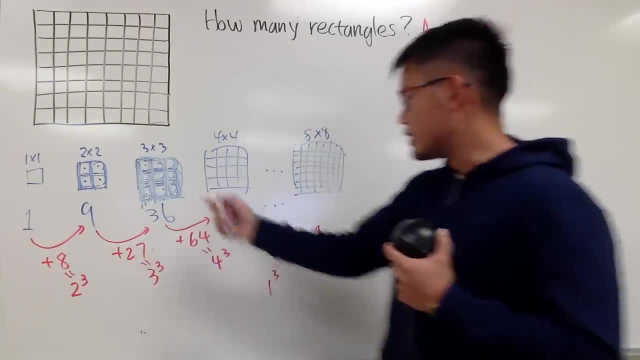 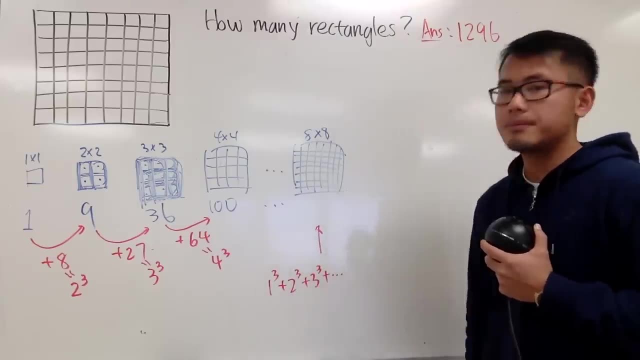 And then, each and every time, you just do two to the third power, three to the third power, and so on. So you do one to the third power, plus two to the third power, plus three to the third power, plus dot dot dot. 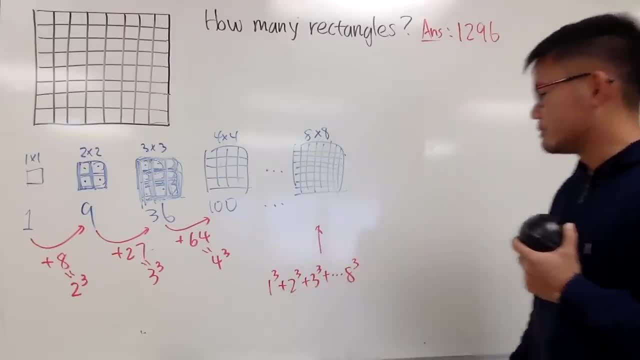 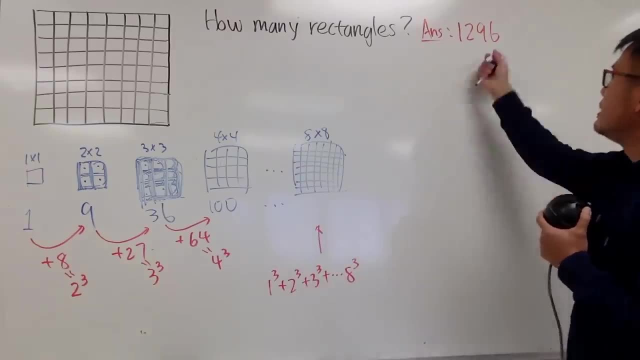 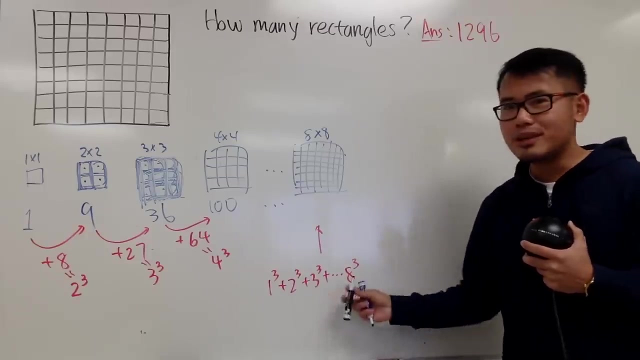 Up to eight, to the third power, And by now, if you have a calculator, you can just, you know, type this onto the calculator and you'll see the answer is 1296.. And now some of you guys might be mad at me, because I'm still counting right. 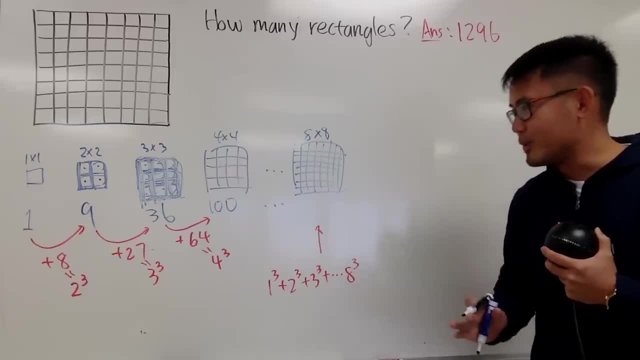 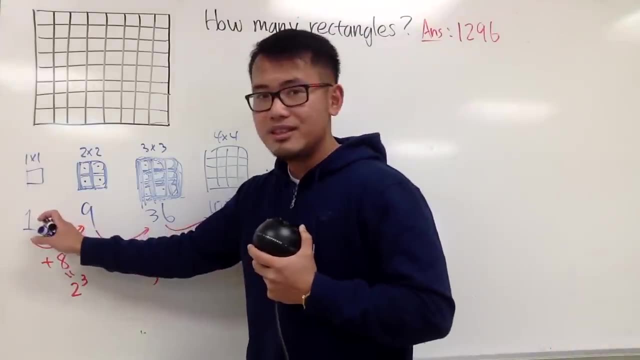 So that's not efficient at all. Don't worry, I'm going to help you. I'm going to make this so cool for you. okay, Look at, this is one which is the same as one squared. Oops, sorry, wrong color. 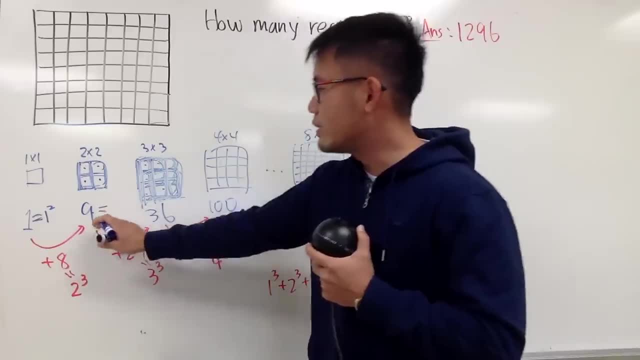 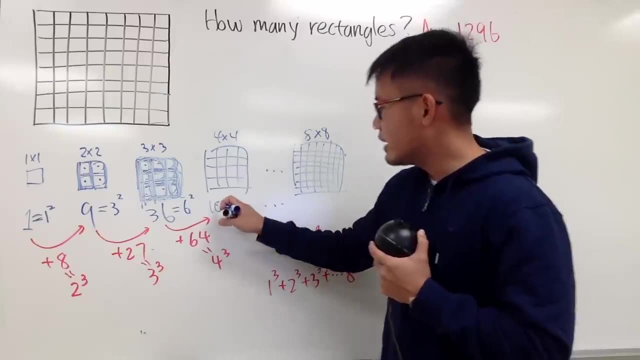 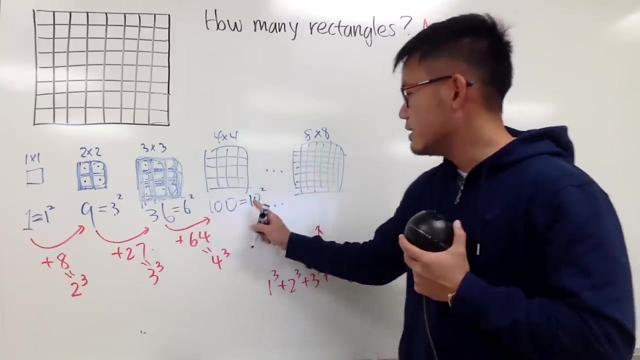 One squared, And if you look at nine, this is three squared. If you look at 36,, this is six squared, And if you look at 100, this is ten squared. And look at one, three, six, ten. 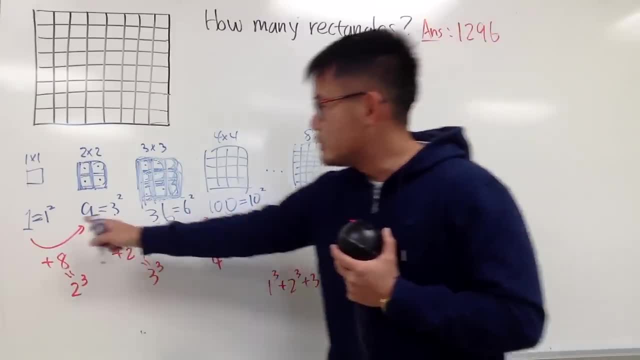 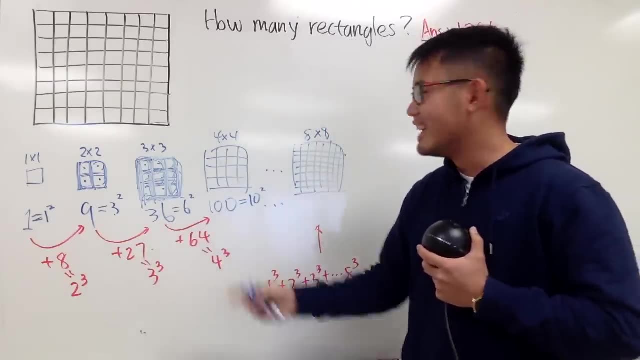 Can we figure out the pattern for the next one? If you just look at the base, from one to three is you add two. From three to six, we add three. From six to ten, we add four And you can imagine. the next one is just that. 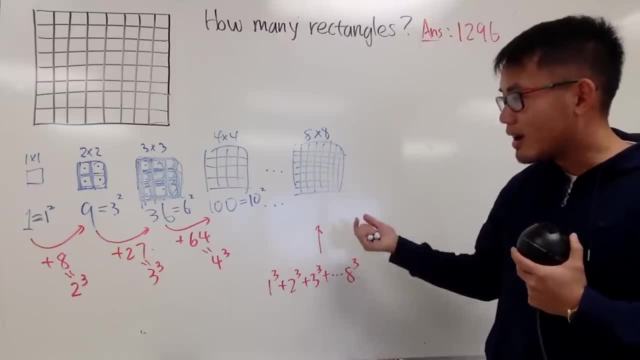 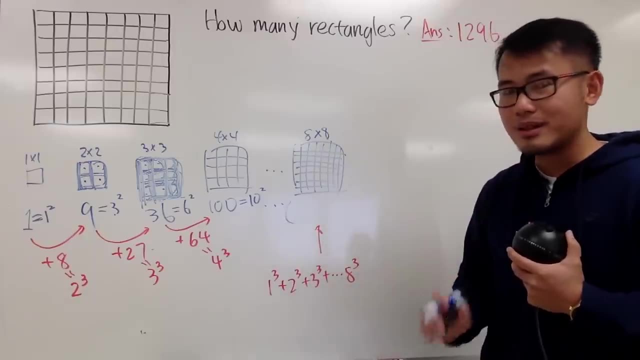 We add five and so on, right. So in fact, here, once we have the eight by eight situation, we could have done the following: This right here, it's the same as saying: let me just write this down again. 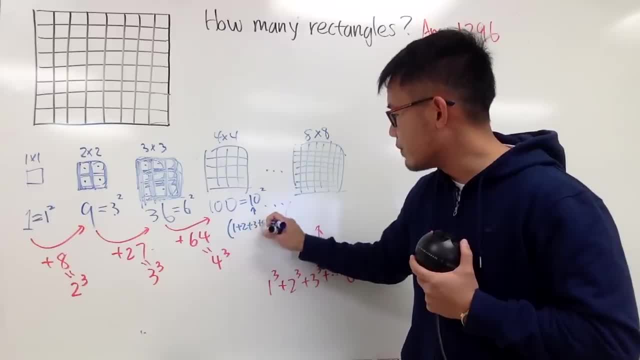 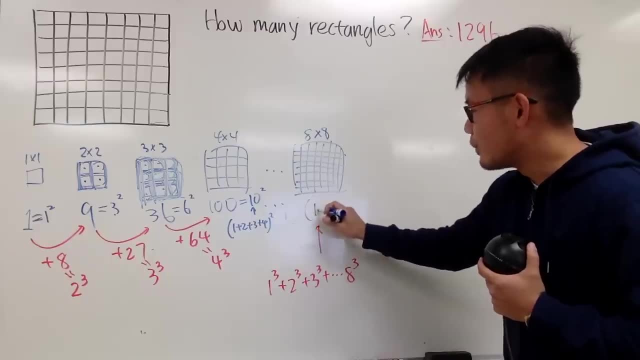 the ten squared is the same as saying one plus two plus three plus four squared right For the eight by eight situation. this right here, it's the same as one plus two plus three plus four squared right. And this right here it's the same as one plus two plus three plus four plus five plus dot-dot-dot up to eight. 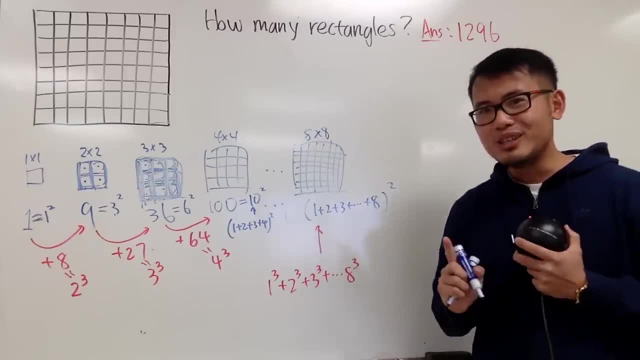 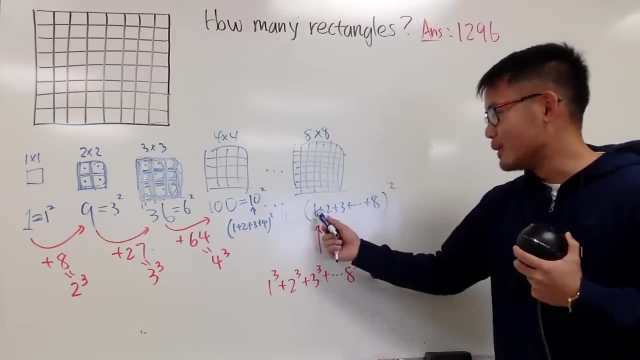 and then you square that. And now I just showed you, guys, a really cool formula where you want to find the sum of the cubes. In fact, you need to know the sum of the first natural numbers and then you just square the result, that's all. 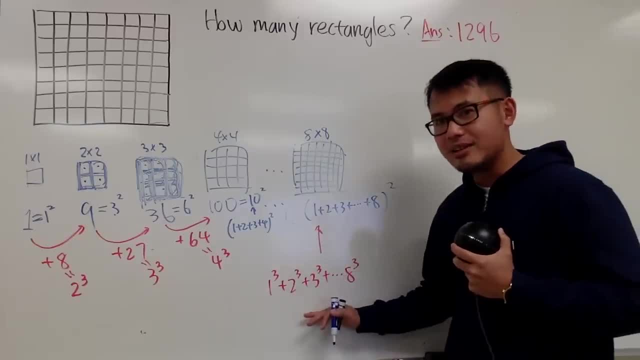 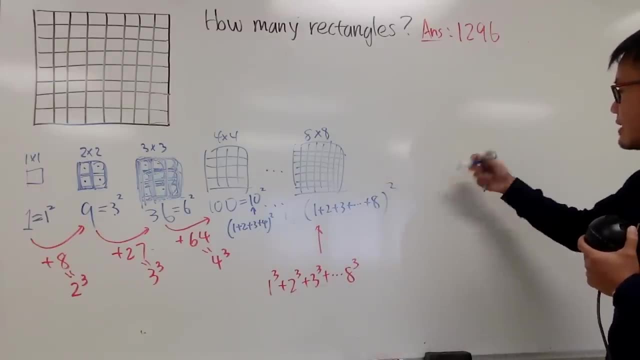 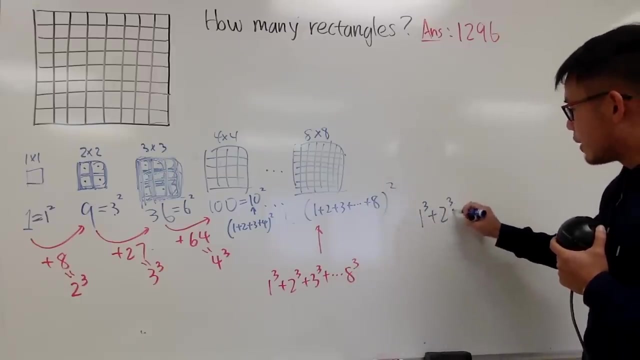 So the idea is that this is counting how many rectangles that we have. so it's this: They must be equal, right? Here's a really nice bonus. It's like the icing on the cake. Let me write this down: When we have 1 to the third power plus 2 to the third power, plus dot, dot, dot, plus n to the third power, 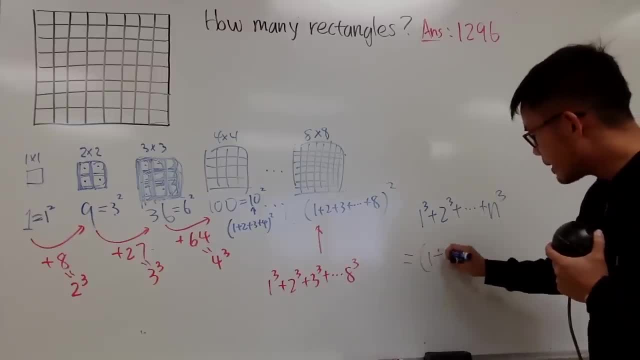 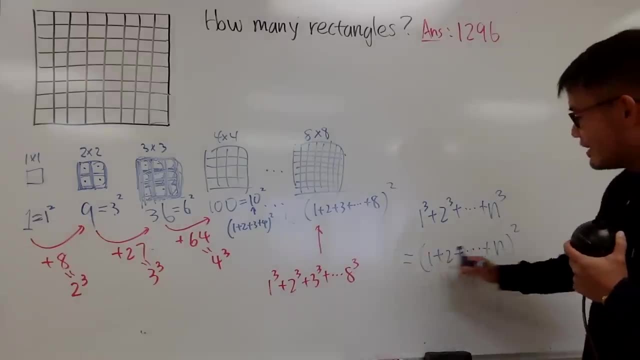 this right here is equal to 1 plus 2 plus 3 plus 4 plus dot dot dot plus n, and then you square the result. And didn't we do this already with five different ways? Yes, we did So all this right here. you can watch my other video for it if you haven't. 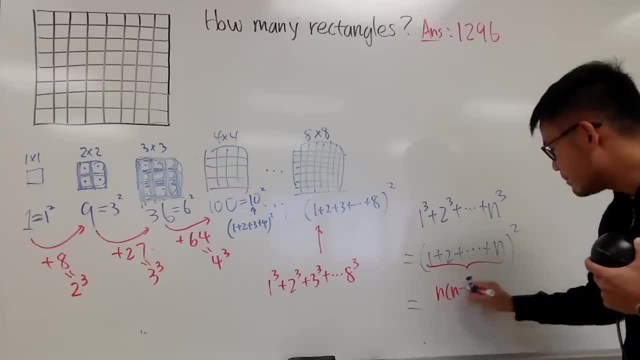 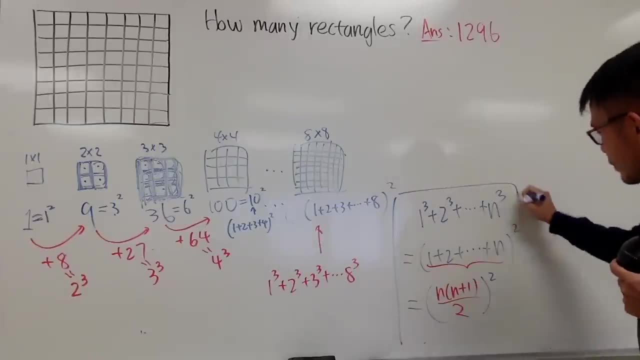 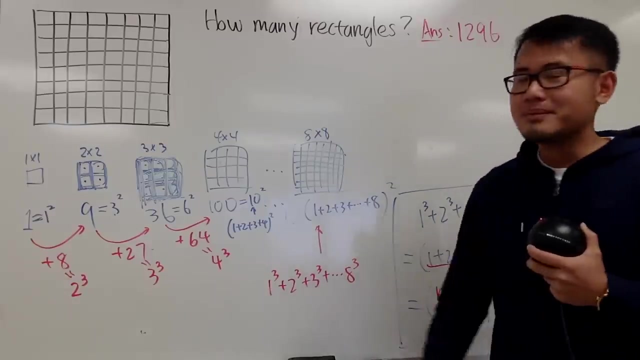 It's equal to n times n, plus 1 over 2, and then to the second power. So this is a nice way to argue that. how to find the sum of the first n cubes. Okay, as I said, this is still not the best way to do this. 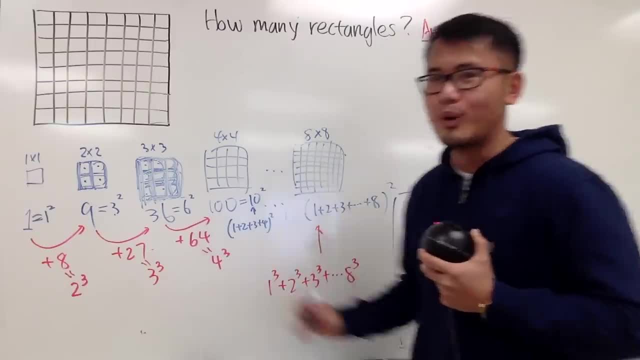 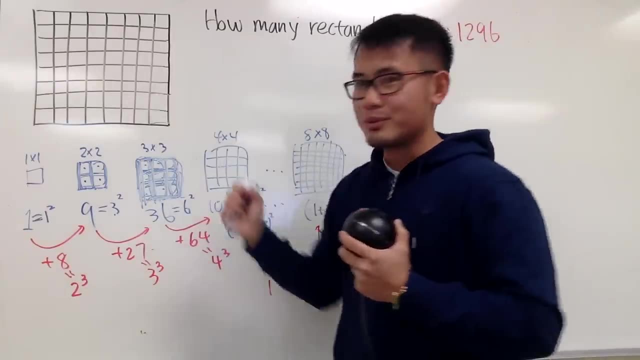 Now, let's do this again. Let's do some combinator, which is one of the best in the world right Now. go back to the big picture. Let's do the big thing right now. right, We're all adults now, so we can handle this. 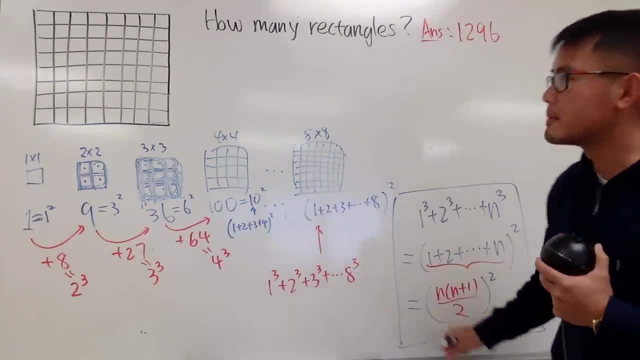 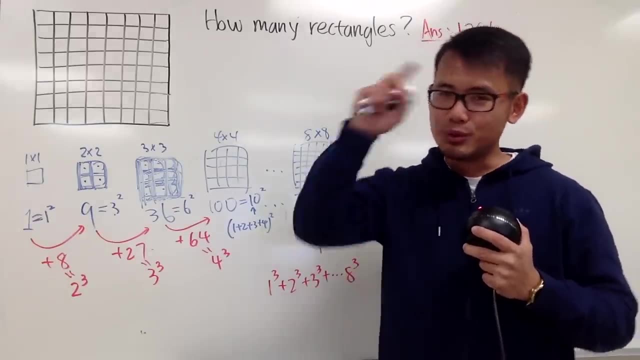 We don't need to look at the small cases, right? Let me show you how to do it. Okay, what makes a rectangle a rectangle? Of course, we must have two sides on the top. one side on the top, one side on the bottom. 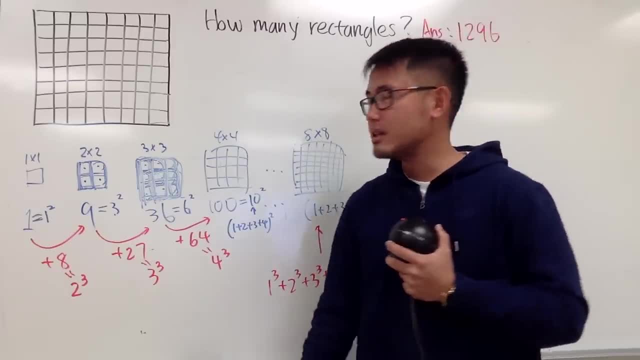 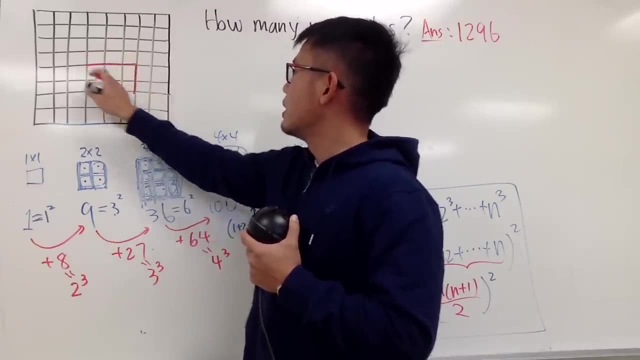 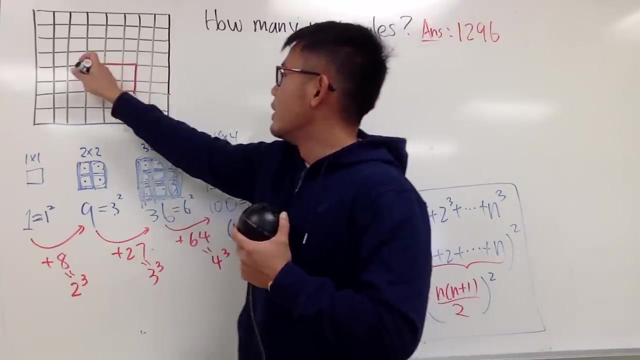 and then two sides, one on this side, one on the other. Let's say, if I pick this rectangle from this board, which is a 3x2 situation, it has four sides, of course, And remember, as I said, we have one side here on the top, one side right here on the bottom. 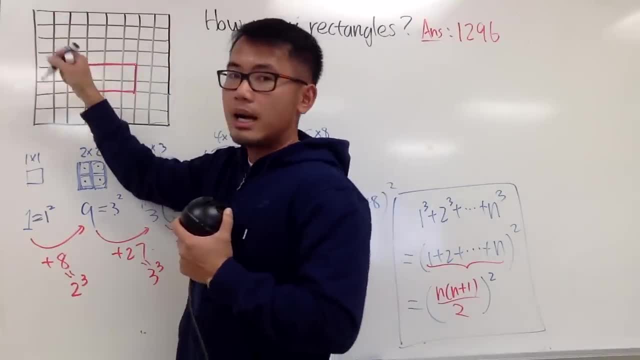 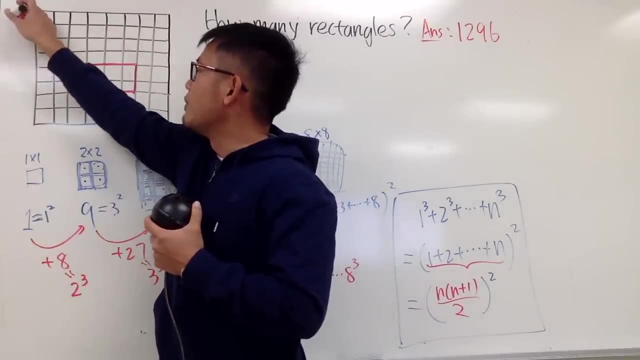 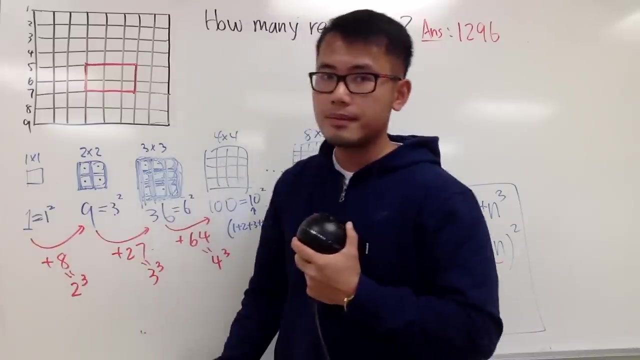 Now you see right here on the side how many horizontal lines do we have. You can just well nine lines, but I will label it for you: One horizontal line, two, three, four, five, six, seven, eight, nine. 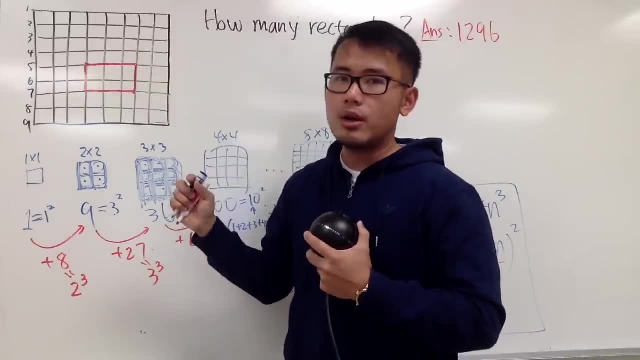 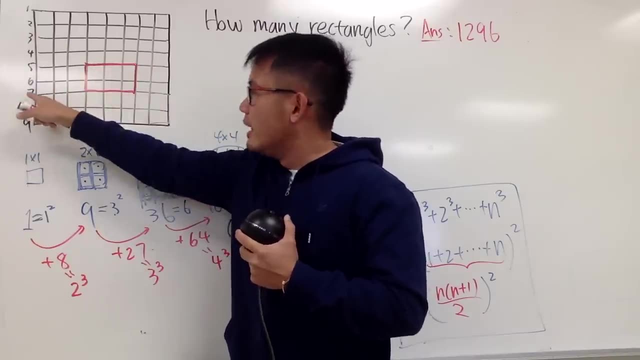 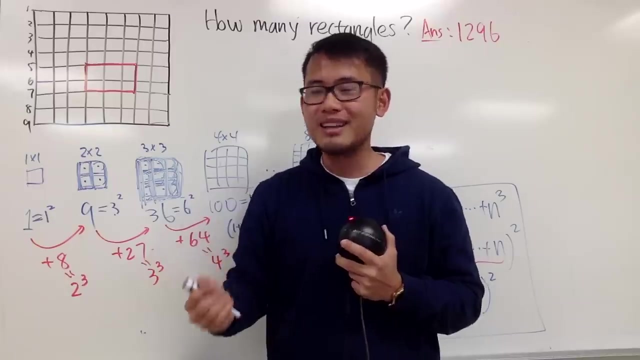 So you see, if you want to select this as your rectangle, what we did is we chose line number five for the side to be on the top and then line number seven for the side to be on the bottom right. And how many ways can we choose two lines out of a total of nine? 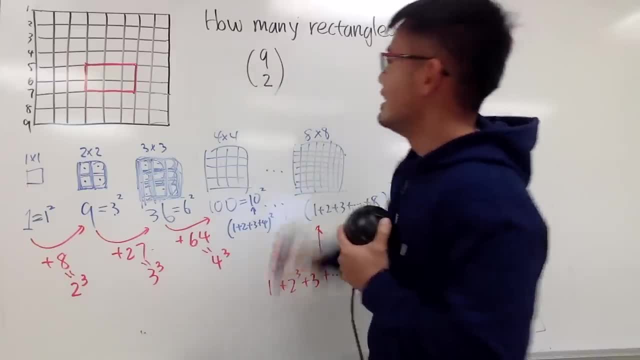 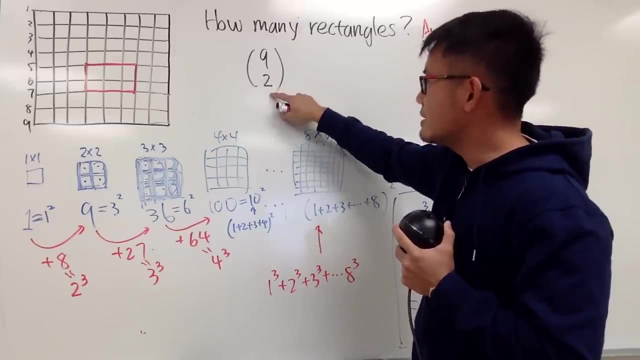 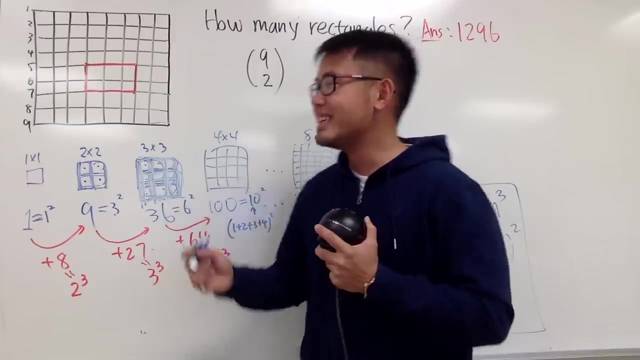 That's precisely nine choose two, isn't it? Nine choose two tells you the number of ways that we can choose two things out of a total of nine things. right, So that's good. And now how can we select these two sides? 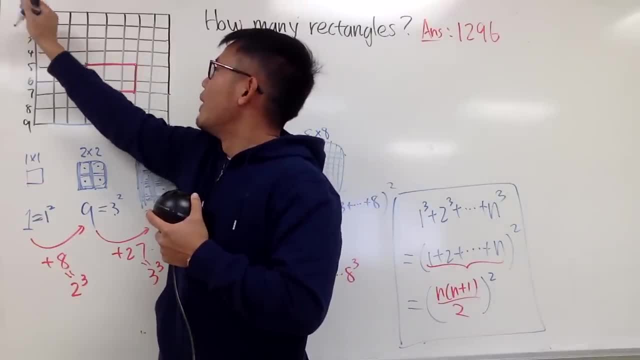 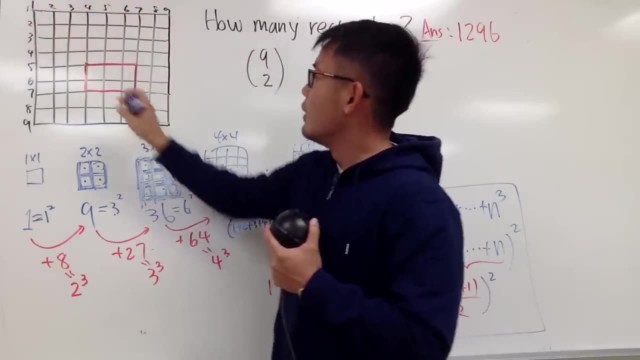 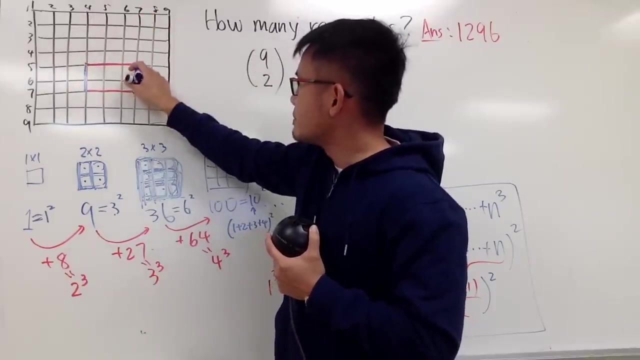 Well, same argument Right here we have one, two, three, four, five, six, seven, eight, nine lines as well. We just chose line number four to be the side on the left And then line number seven to be the side to be on the right. 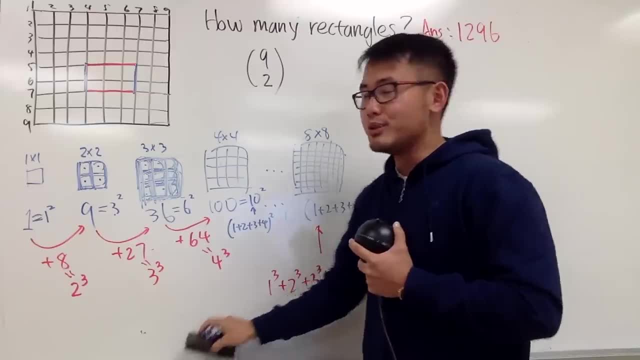 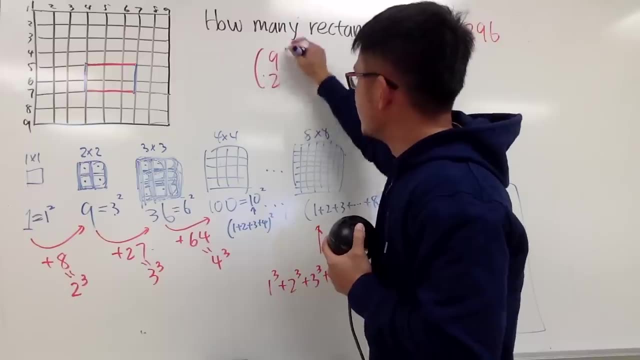 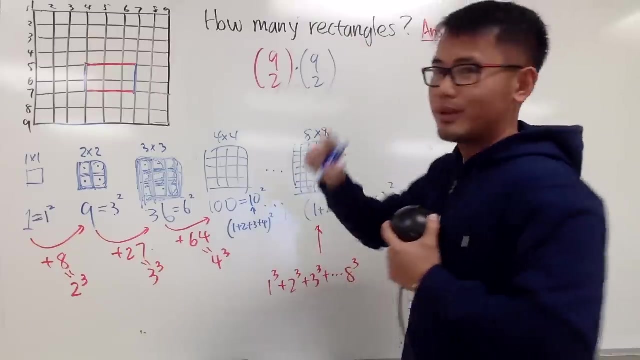 And guess what? Yes, we still have the nine choose two. So let me do this. actually, My color was actually not matching This. right here is nine choose two. right For the top and bottom, And then we multiply by nine: choose two for the left and right. 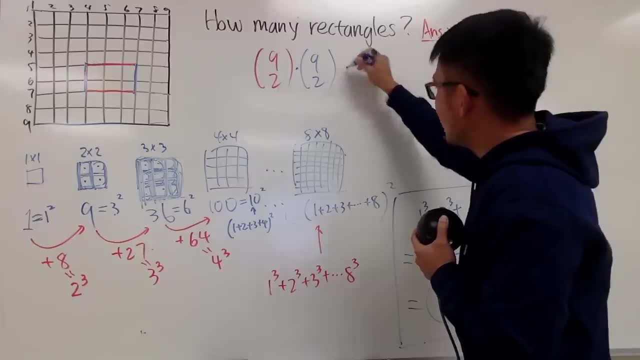 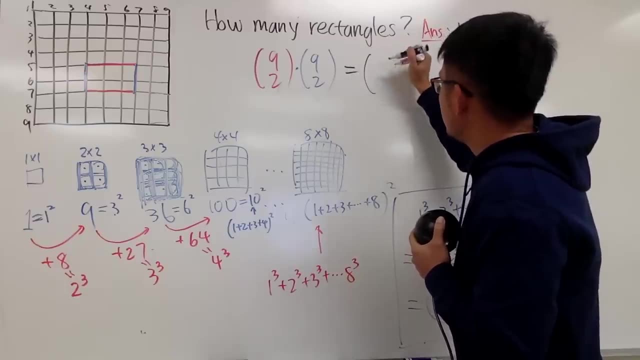 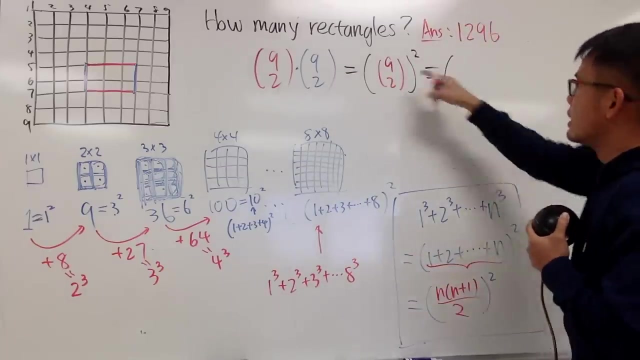 So in another word, this right here is nothing but just nine choose two squared. So I'll write this down for you guys: This is just nine choose two, and then we square that And nine choose two. if you would like, you can do it like this: 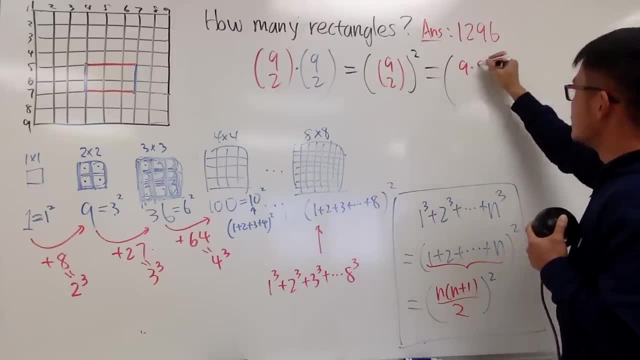 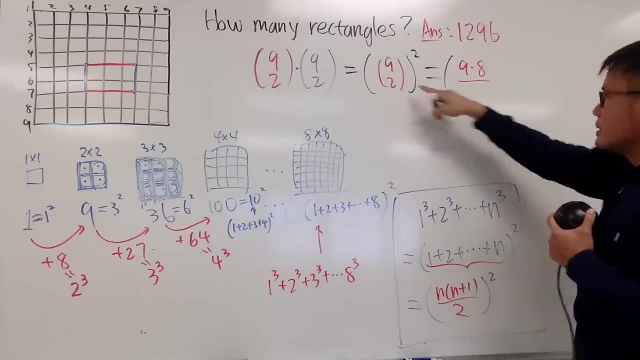 Just put down nine, multiply by the next number, which is eight, and you stop. You just need two terms, because you have the two. Now it's a division. This was not division, right? There's no fraction part here, all right. 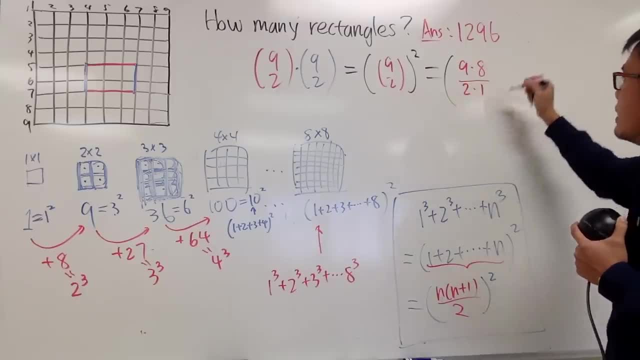 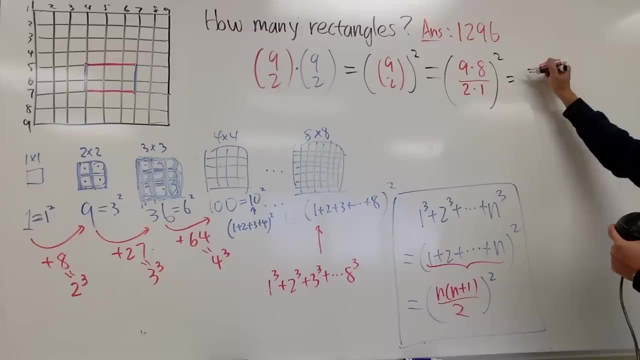 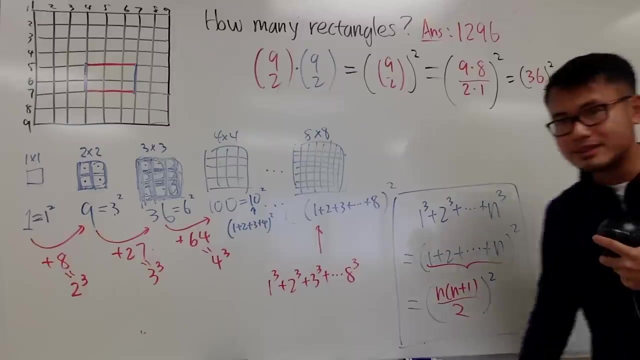 On the bottom. you just divide by this factorial, namely two times one, And you can work this out now: Nine times eight is seventy-two. divided by two is thirty-six, So you have thirty-six squared and you end up with one thousand two hundred ninety-six. 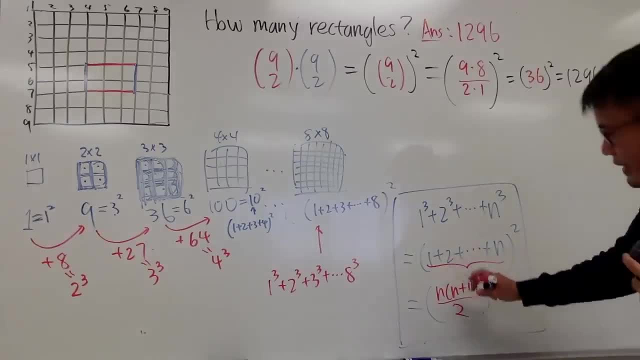 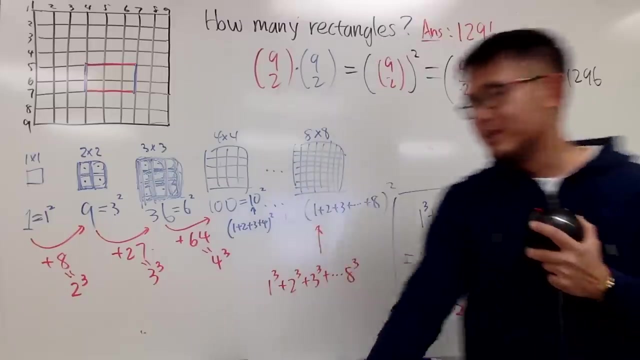 All right, And yes, this right here. I also showed you that one plus two plus three plus dot dot dot plus n, it's precisely equal to n plus one. choose two. Same exact argument. You can watch my previous video for a detailed argument, though.